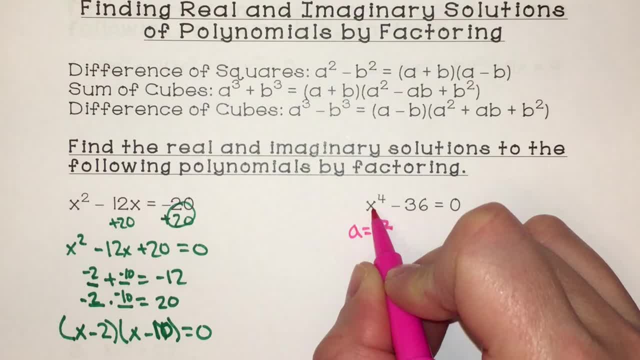 x to the fourth minus 36 is equal to 0.. So I'm going to use the difference of squares- So I know that x squared times x squared is x to the fourth- To figure out what b is. I know, 6 times 6 is 36.. So 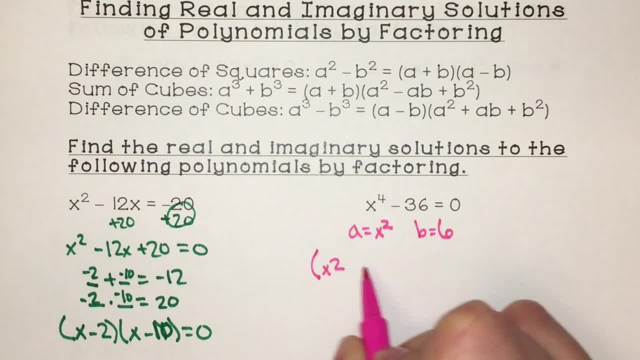 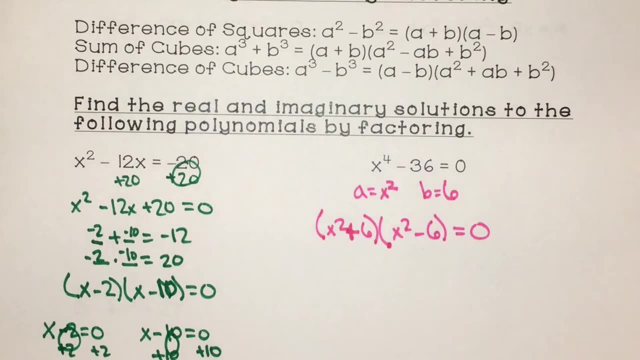 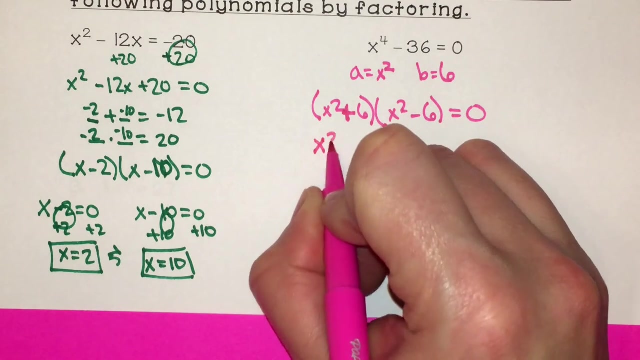 we have x squared plus 6 times x squared minus 6 is equal to 0.. Okay, and all I did was use the difference of squares. Okay, so now I'm going to set each of those individually equal to 0.. We have x squared plus 6 equals 0.. And over here. 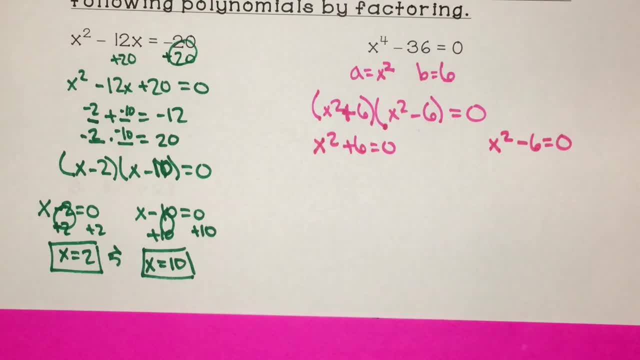 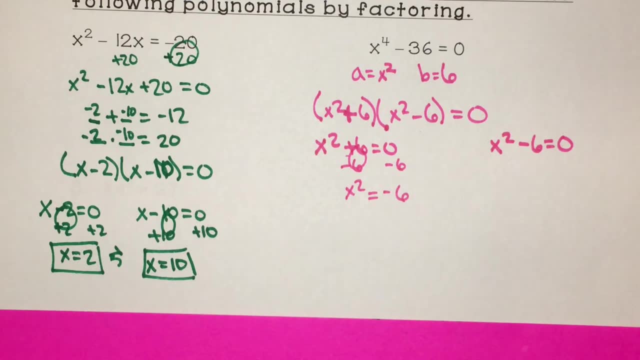 I'll do: x squared minus 6 equals 0.. First thing: subtract 6 on both sides to get x squared equals negative 6.. But I know what, want to know what x is not x squared. So I have to take the square. 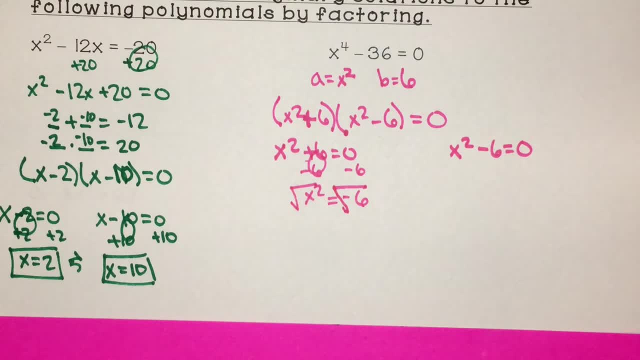 root of both sides. But anytime you're taking the square root of a squared value, well, you squared something. you don't know if it was originally positive or negative, So we're going to have to take that into account. over on the side, Square root of x. squared is just 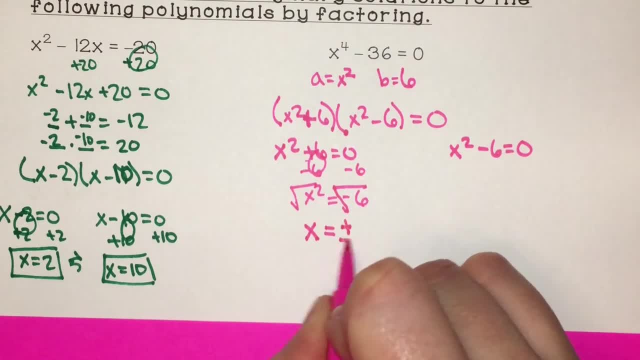 x. They undo each other, So we have to take into account whether it was originally positive or negative. All right, square root of negative 6.. Well, I can't factor 6 in, because 2 times 3, I don't have anything multiplied by itself that I can factor out, But it's multiplied by negative. 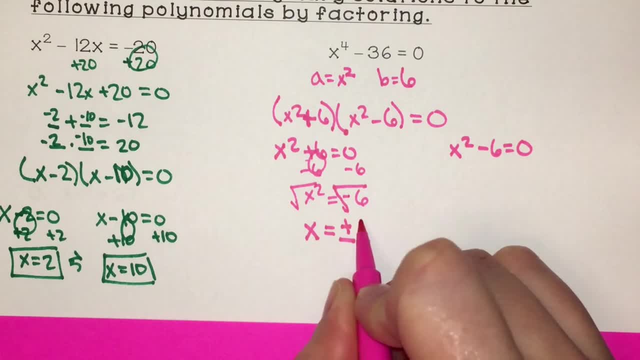 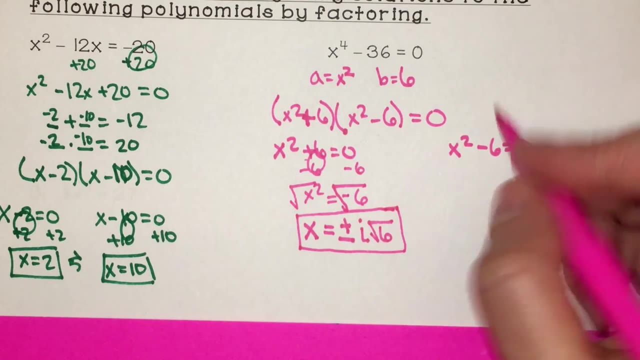 1. So when we factor that out, we get an i And it's left with a square root of 6.. So there are two answers here: x equals positive i times the square root of 6, and negative i times the square root of 6.. Okay, so let's do this one. 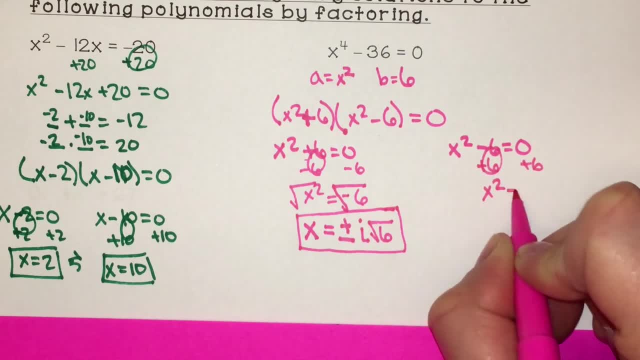 We're going to add 6 to both sides and get x squared equals 6.. Again, we want to know what x is. So take the square root of both sides. Square root of x squared is x. We have to take into account both positive and negative, because when we square root of x squared we get an i. So we're 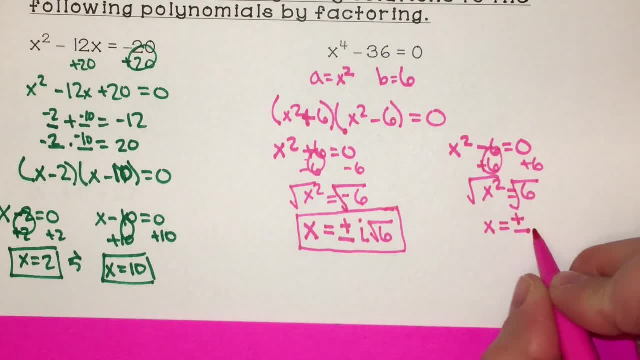 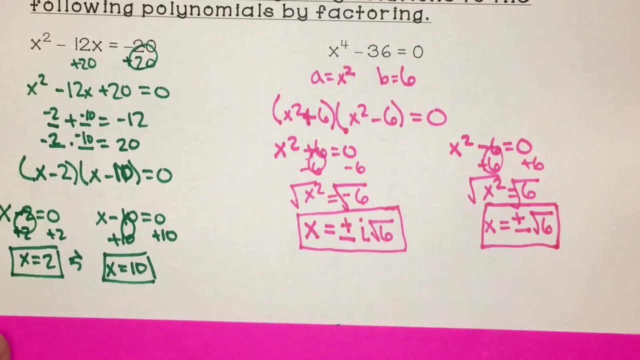 going to add x squared. It could have been either. And square root of 6 cannot be simplified, It is as simple as it can get. So x equals square root of 6 and negative square root of 6.. So there are four answers altogether for this one polynomial. All right, so let's try something a little. 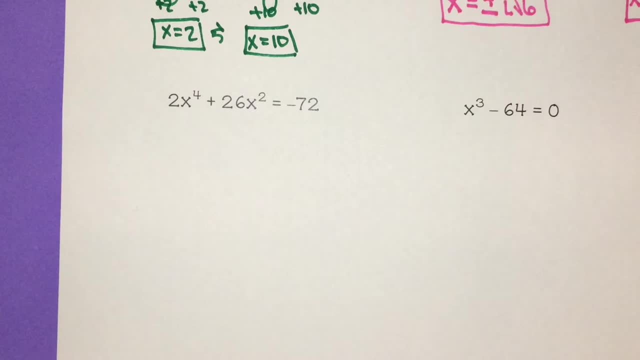 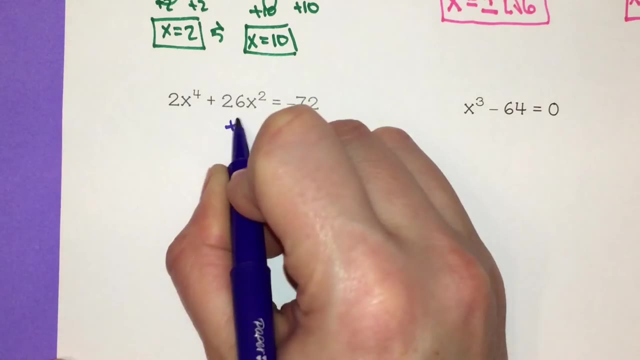 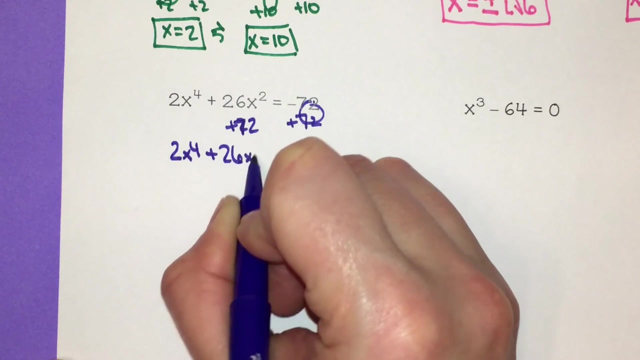 different On this one. let's see, we need to get everything moved to the left. So I'm going to add 72 to both sides, So we get 2x to the 4th plus 26x. squared plus 72 is equal to 0.. 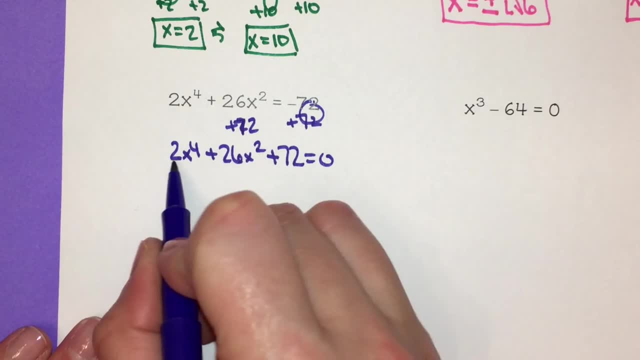 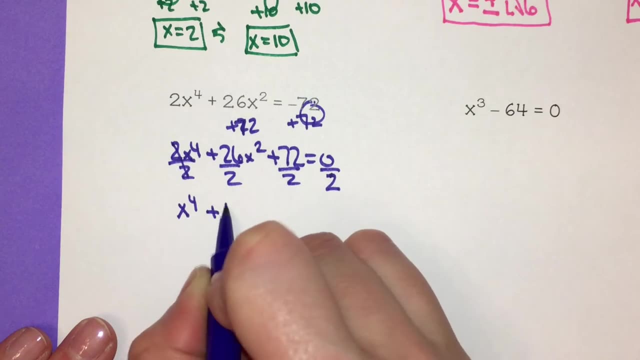 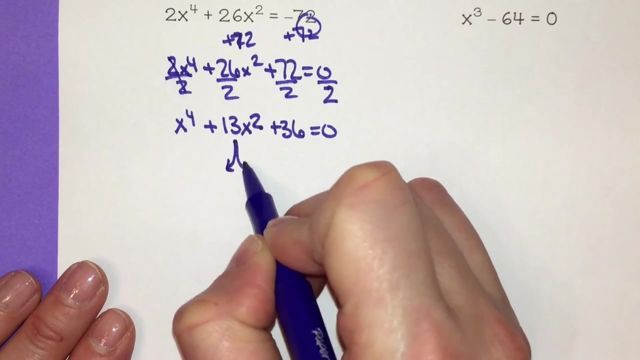 All right. so first thing I'm going to do is divide everything on both sides by 2.. 2 divided by 2 is 1.. So we have x to the 4th plus 13x, squared plus 36. Is equal to 0.. Okay, I need to split this middle into 2.. I need to figure out what I can split it. 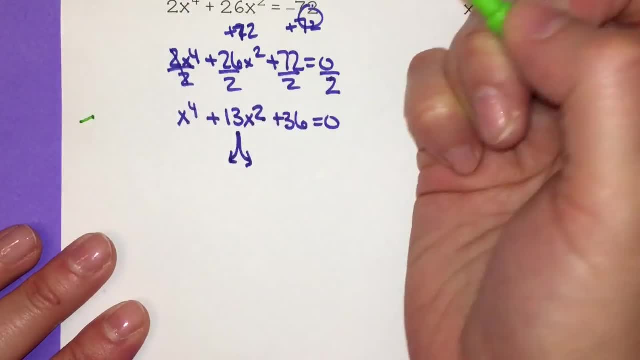 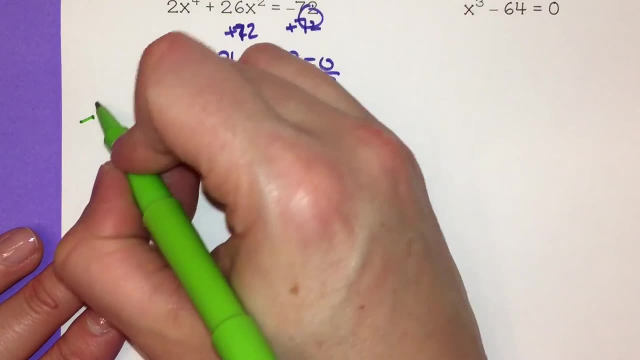 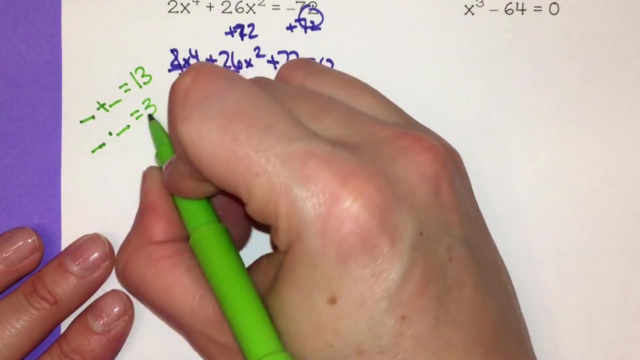 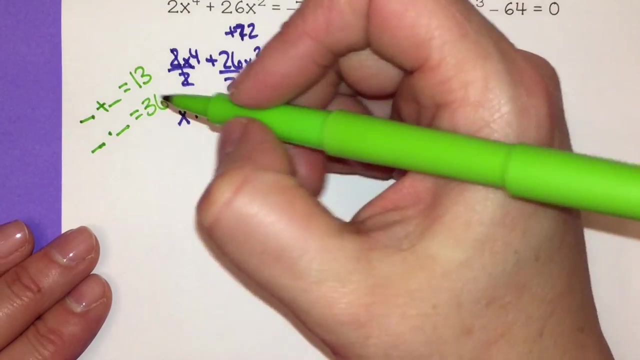 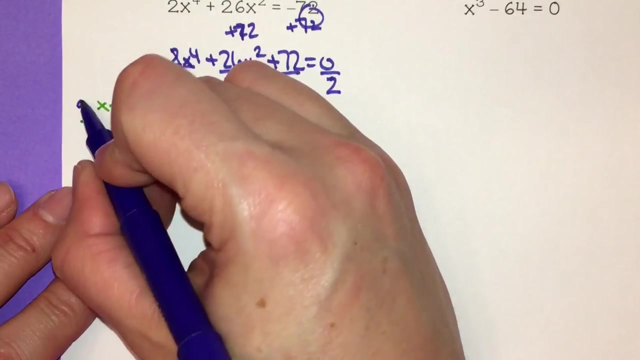 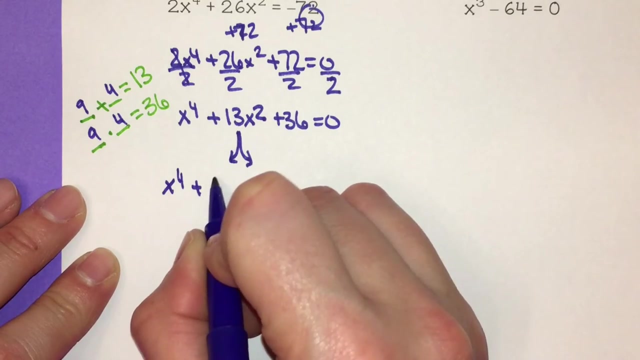 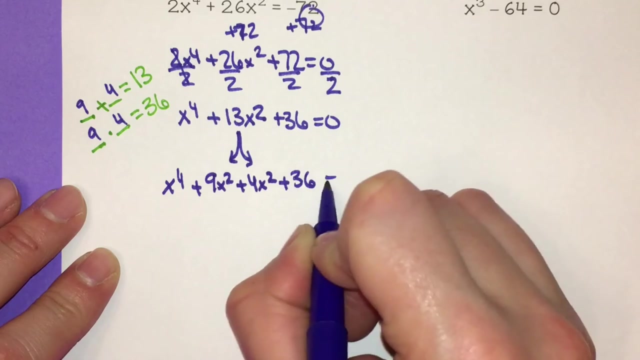 into. So I have to determine what plus what. or let's see what plus what equals 13 and what times. what equals 36.. Okay, so we have 9, and 4 should give this to us. So we have x to the 4th plus let's do 9x squared plus 4x squared plus 36 is equal to 0.. 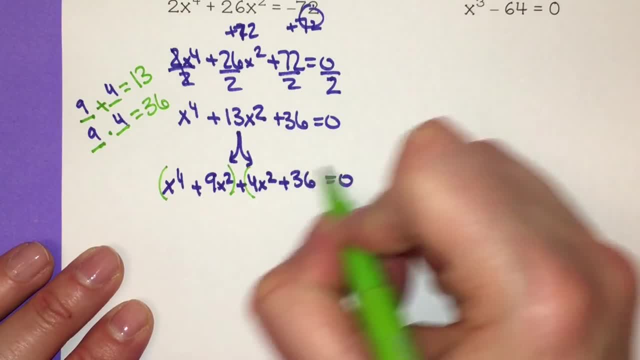 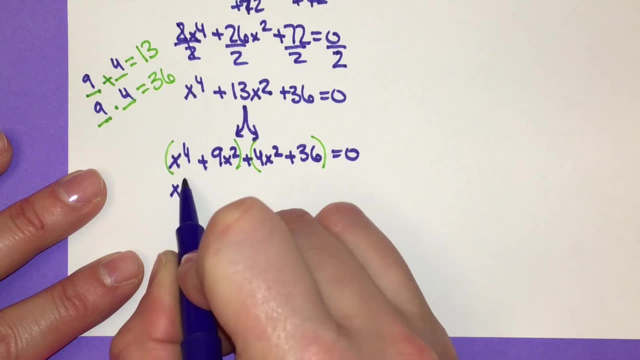 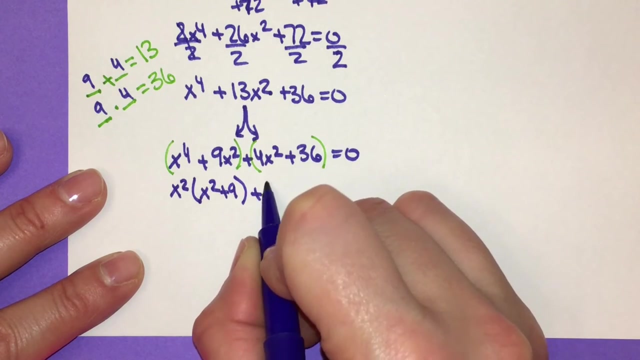 Okay, so I'm going to put parentheses around my first two and then around my last two terms. I can factor out of this first one x squared, and I'm left with x squared plus 9 plus the second one. I can factor out a 4 and I'm left with x squared. 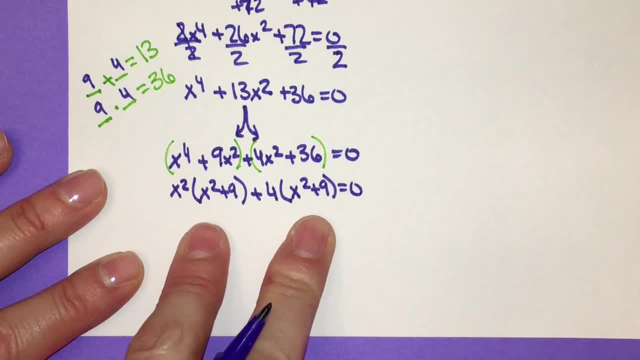 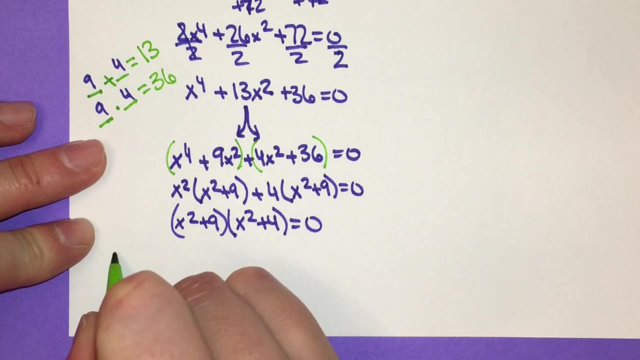 plus 9.. Okay, factor out that greatest common factor of x squared plus 9, and it's multiplied by x squared plus 4, is equal to 0.. All right, so on this, I have to set each of these individually equal to 0.. So x squared plus 9 equals. 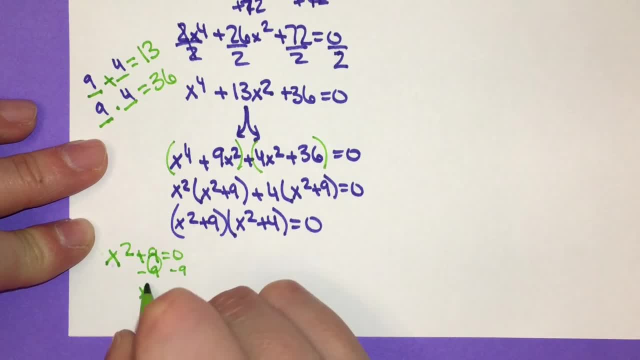 0. subtract 9 on both sides and we get x squared equals negative 9.. Take the square root of both sides. we get x equals positive and negative, negative. well, the square root of 9 is 3, because 3 times 3 is 9, but we do have that. 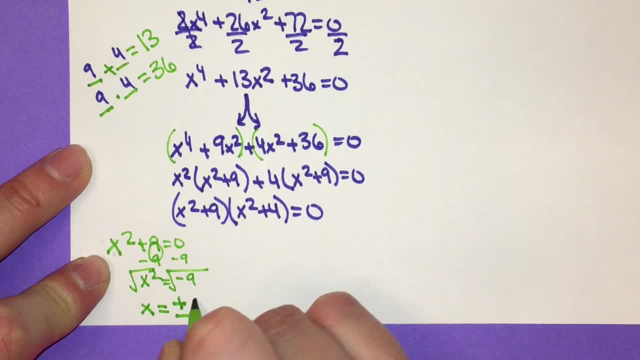 negative. so it has to come out as i. so we have positive and negative 3i. Also, we have to do: x squared plus 4 equals 0, so subtract 4 on both sides, we get x squared equals negative 4, take the square root and we get x is equal to. again, take into account positive and 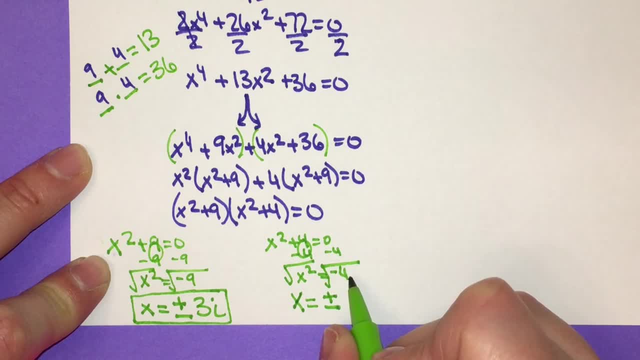 negative. alright, square root of 4 is 2, because 2 times 2 is 4, and square root of negative 1 is i. so we have 2i, Okay. so on this one we do have 4 answers, Alright, let's. 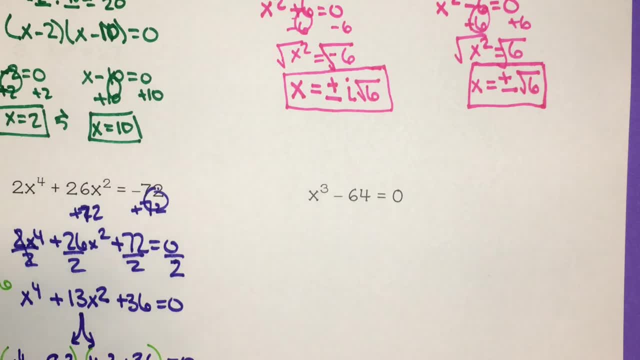 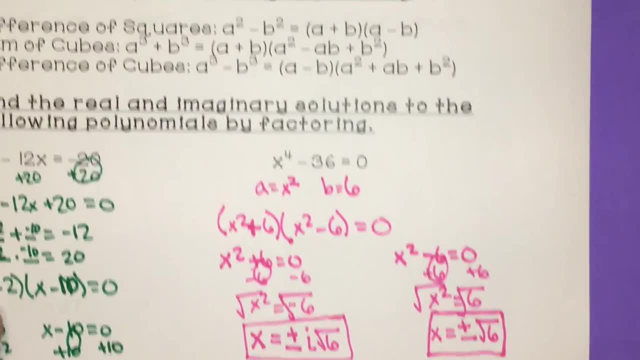 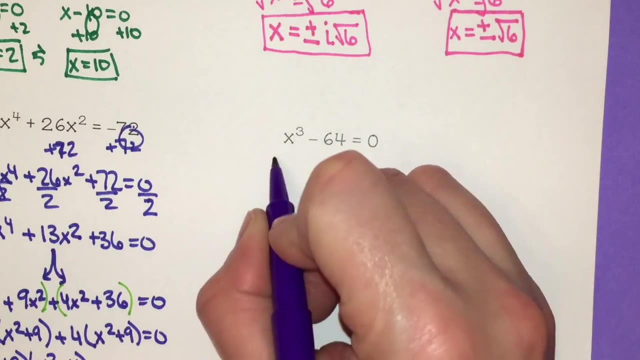 try this last one together, and then I'll let you try some on your own. Alright, so we have x cubed minus 64 equals 0, so this is a difference of cubes. so we want to use this formula. So the a value is just x, because, well, what number times. 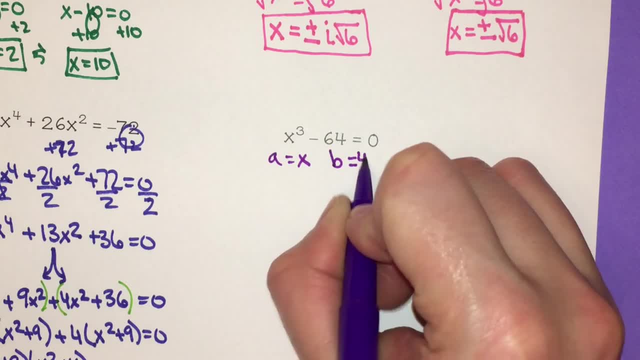 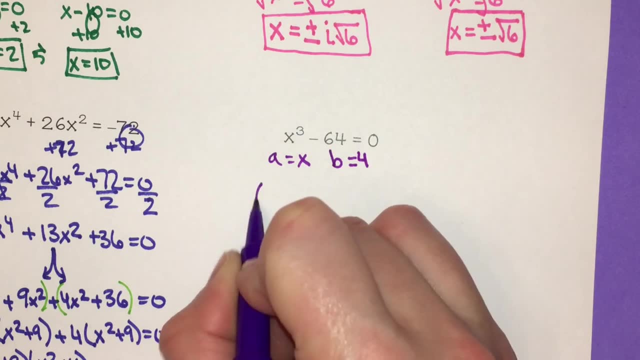 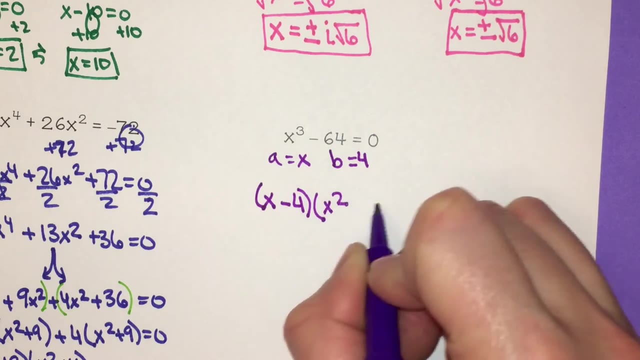 itself 3 times is x cubed, The b value is 4, again, what number times itself 3 times is 64? Well, that's 4.. So that gives us x minus 4 times x. squared plus 4 times x is 4x plus 4 squared is 16.. That's equal. 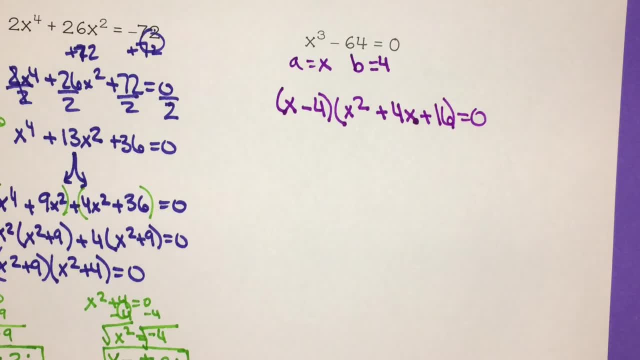 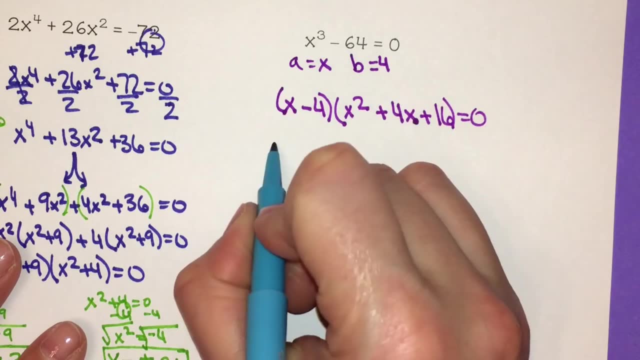 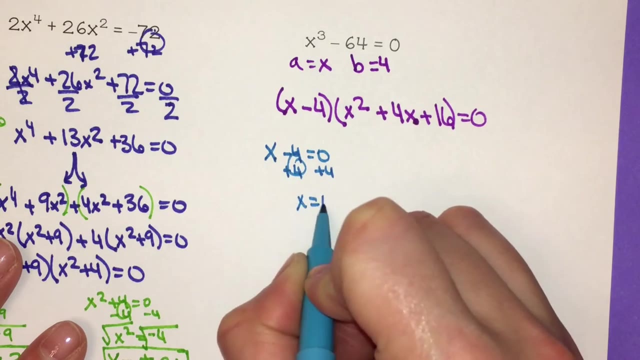 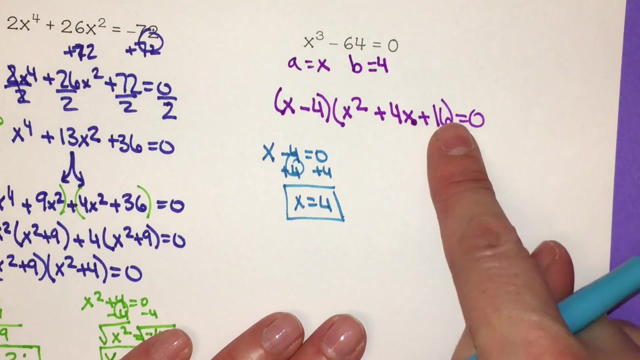 to 0.. Alright, so now on this first one, this first set of parentheses, I can say x minus 4 equals 0, and I'm going to add 4 to both sides. Let's take both squares and say x equals 4, is one of my answers. Okay, over here well. 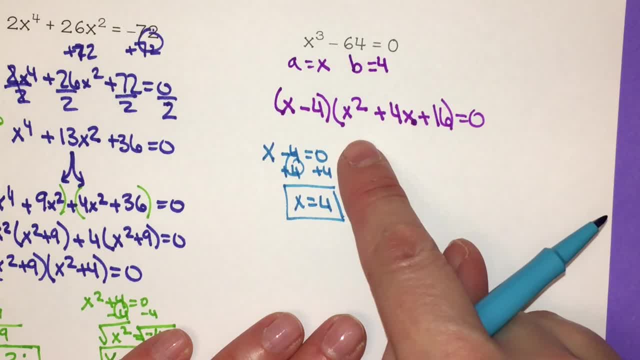 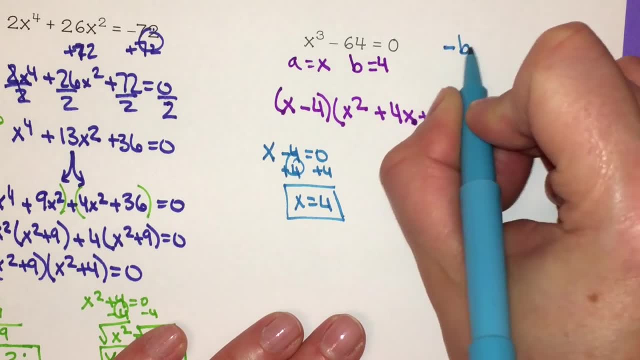 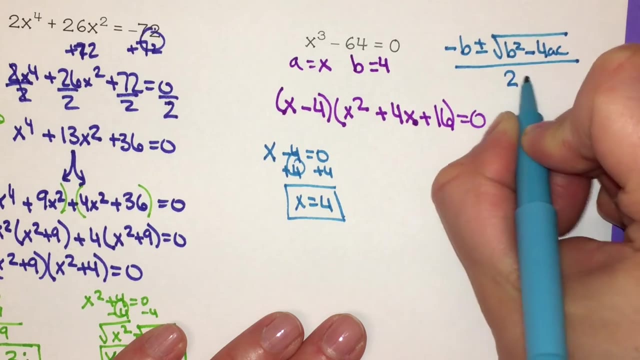 there isn't anything that I can multiply together to get 16 and add together to get 4.. It's not possible, So I'm going to use the quadratic formula Negative b plus and minus the square root: b squared minus 4ac divided by 2a. Okay, so we have x squared plus 16, it form 0.. Let's take two squares together and add 4 to the screen. Yeah, so I need 4 a, so I need 4 c, and then I need 2b and wesmall. So, we have it. Then let's take from square root b times up to 4a, and then then let's say 4a squared and divide it by 2a. Okay, so we have x squared minus 64, so we get x squared minus 64,. so we have x del twoi. 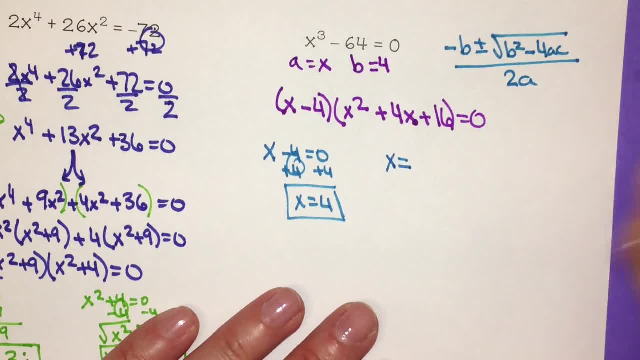 Okay, so we have x equals. well, let's look at: a is 1,, b is 4, and c is 16.. Okay, and if you write it out it can make it easier, so you don't have to put everything in and then simplify. 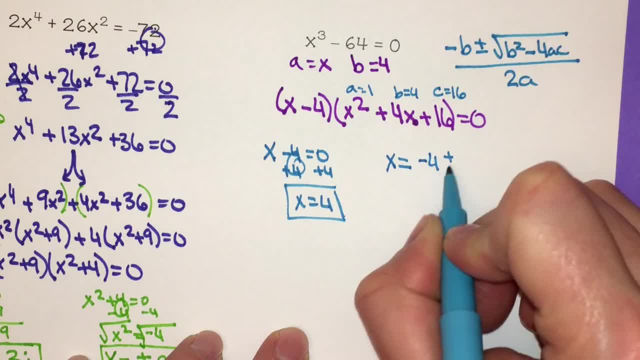 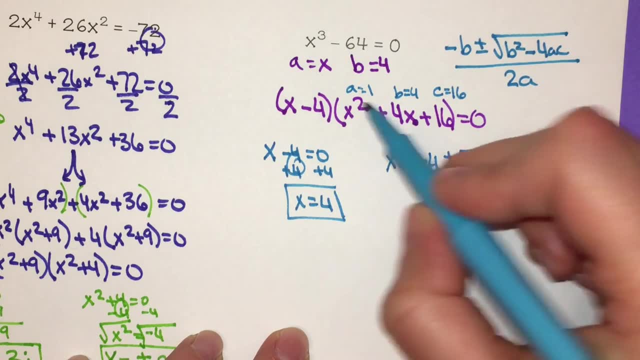 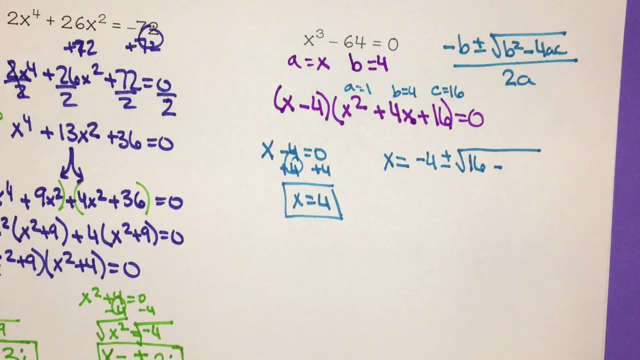 So we have negative b, which is negative 4, plus and minus the square root B squared well, 4 squared is 16, minus 4 times a, 4 times 1 is 4, and 4 multiplied by c, which is 16,, gives us 64.. 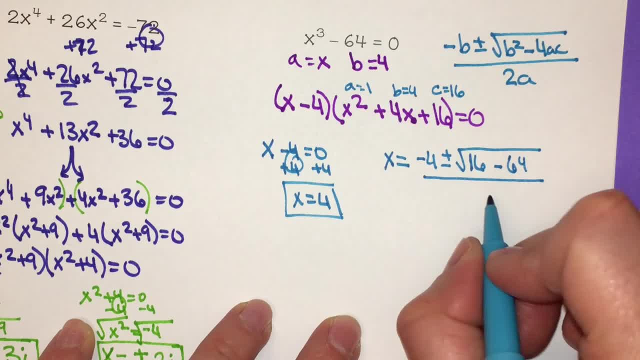 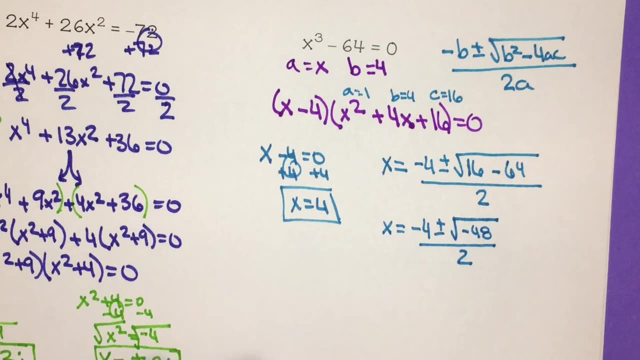 All of this is over 2 times my a value 2 times 1 is 2.. We get: x equals negative 4, plus and minus the square root of negative 48, divided by 2.. Okay, so 48,. if I look at what I can break this down to, I'm just going to do the math down here. 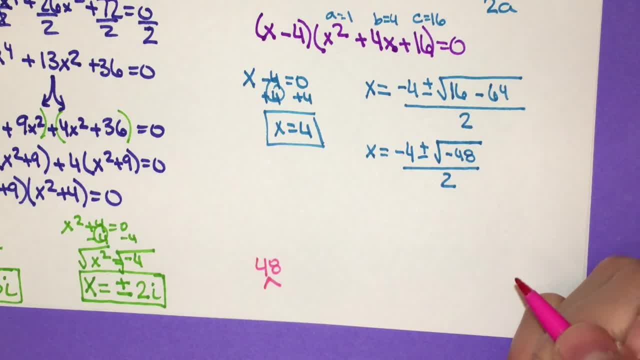 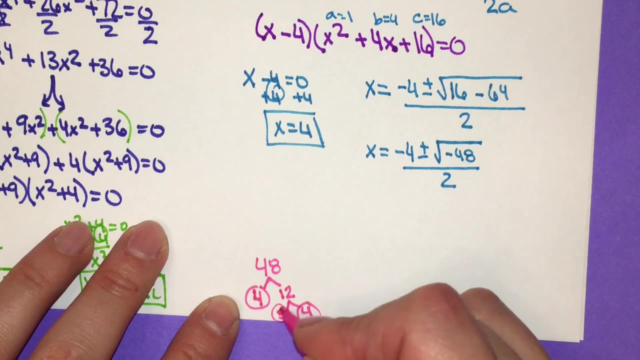 So we have 48,. well, we have. I'm going to do 4 times 12,. 12 is 3 times 4, and I actually don't have to break down my 4s because I do have. I know 4 times 4 can be pulled out. 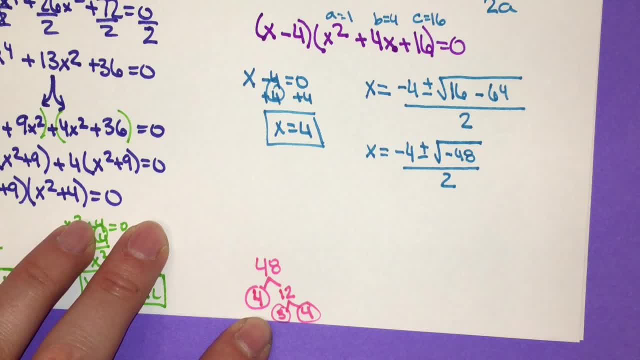 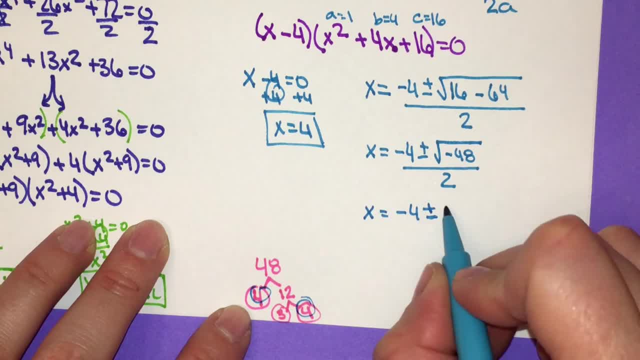 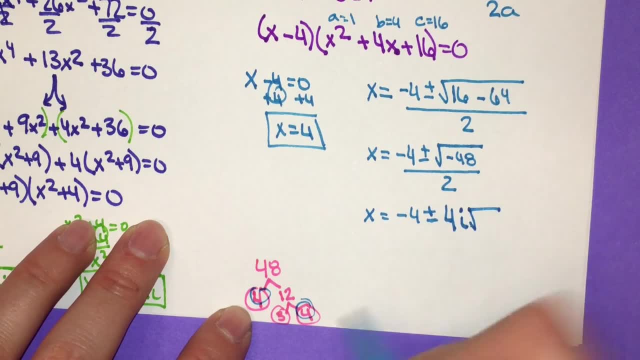 I can pull out this pair of 4s as a 4, and it's multiplied by negative 1, so pull that out as an i and we're left with a square root of 3,. doesn't have anybody to buddy up with to come out. 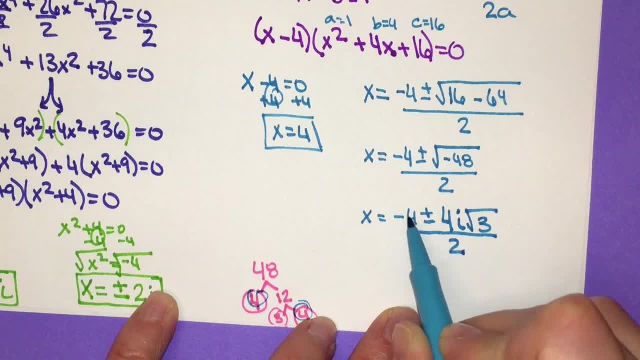 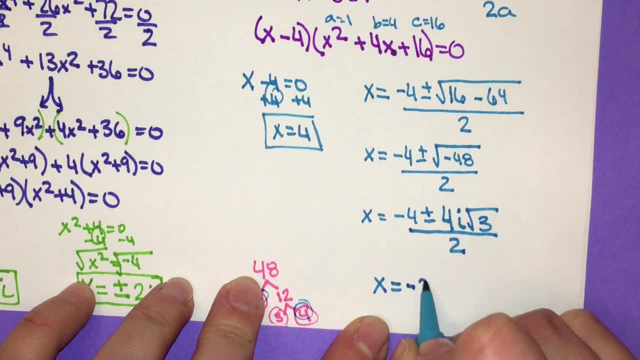 and it's all over 2.. Well, I can divide each of these individually by 2, just simplify it one more time. We have x equals x equals negative. 4 divided by 2 is negative. 2, plus and minus. 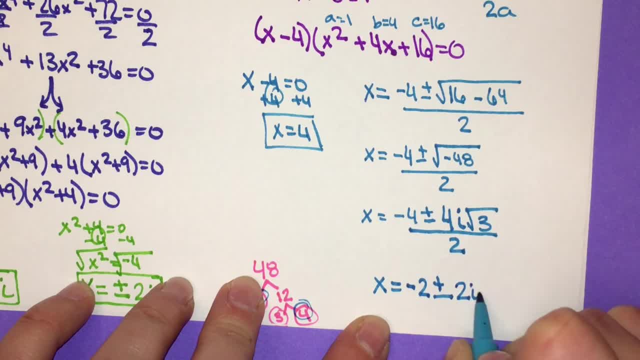 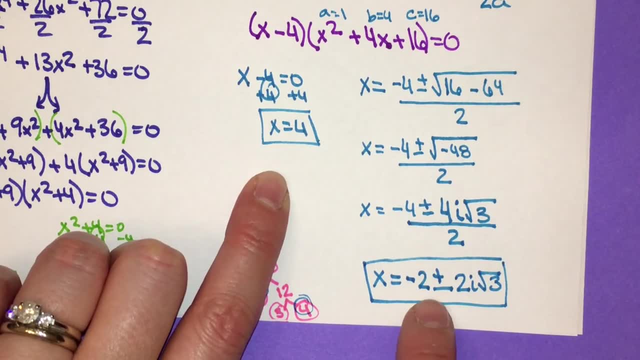 4i times the square root of 3. divided by 2 is 2i times the square root of 3, and so this one has 3 answers, because we have to take into account both positive and negative. Alright, so here are 3 problems for you. to go ahead and try. 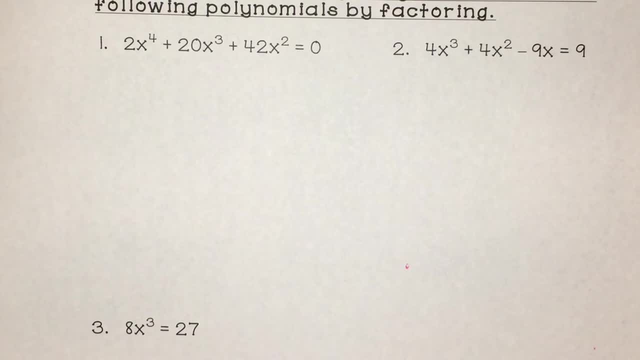 You're going to factor them and when you're ready for the answers, go ahead and pause it here and then come back and we can do them together, Alright, so this first one, First thing I'm going to do is divide everything by 2.. 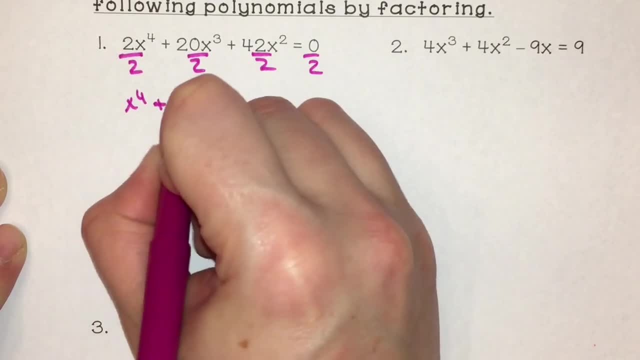 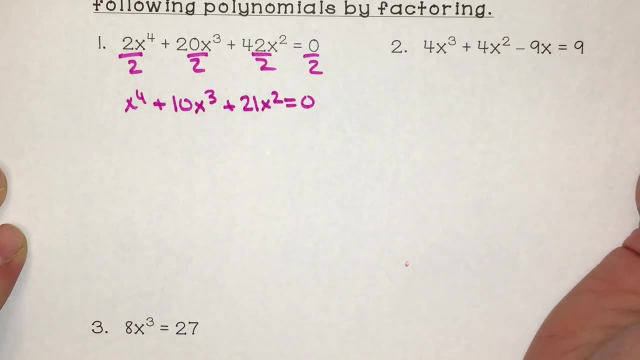 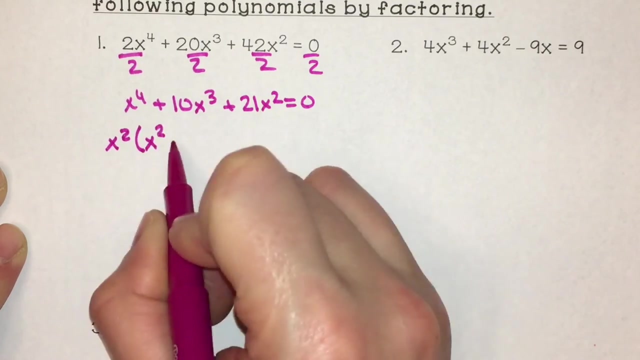 So we get x to the 4th plus 10x. cubed plus 21x squared equals 0.. I can factor out an x squared times. what's left over is x squared plus 10x plus 21.. 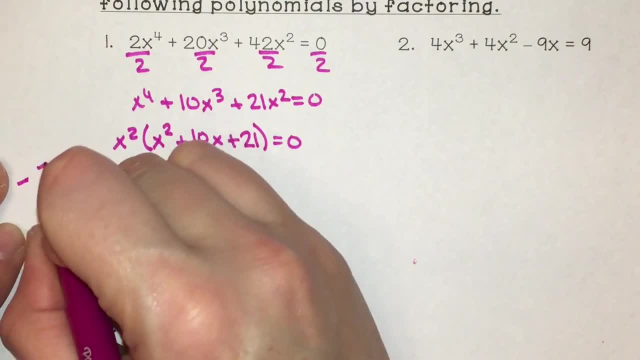 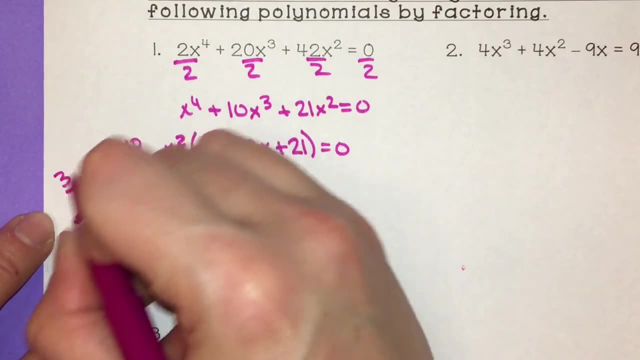 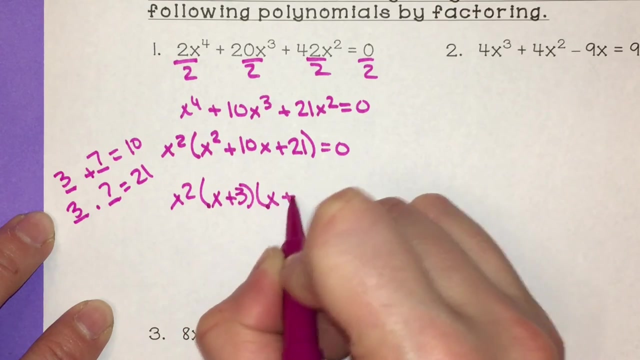 Equals 0.. Alright, so now we have to see: is there anything that we can add together to equal 10, multiply together to equal 21.. 3 and 7 work, So we have x squared times x plus 3, times x plus 7 is equal to 0.. 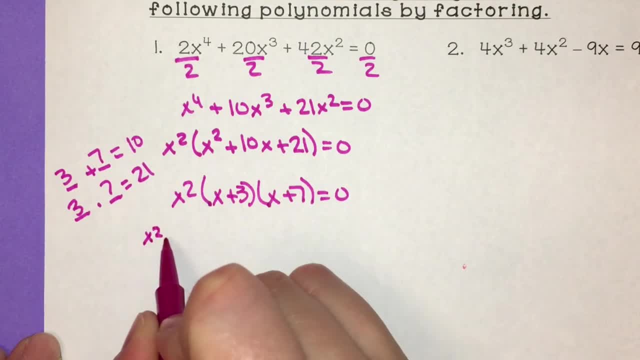 So we have to solve for each individually: x squared equals 0.. x plus 3 equals 0.. And x plus 7 equals 0. zero. Here we have to take the square root of both sides. X equals. well, I don't have to take. 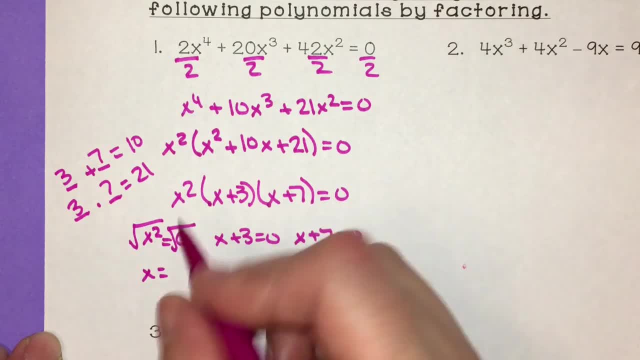 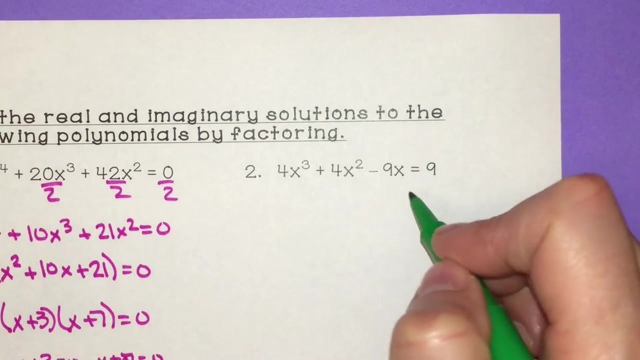 into account positive and negative, because square root of zero is just zero. Subtract three on both sides, and X equals negative three. Last one: subtract seven on both sides, and X equals negative seven. So that one did have three answers. All right, this one Okay. so again, I'm going to 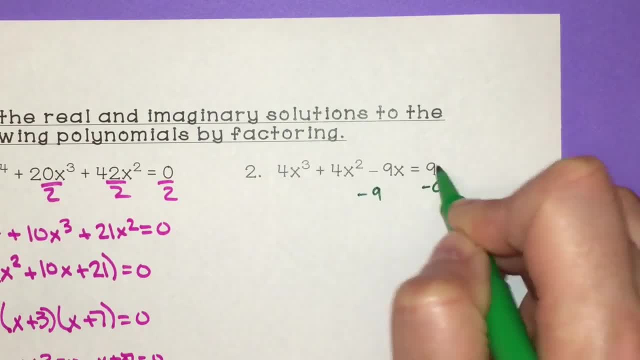 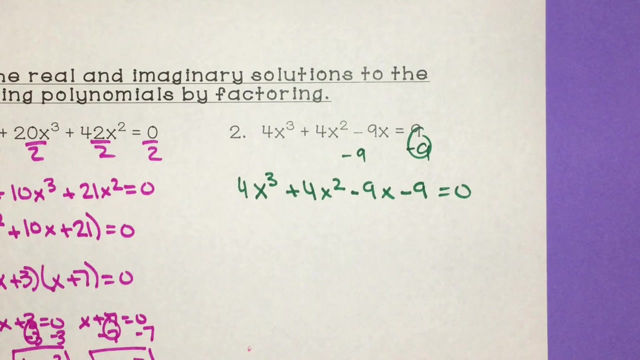 move this nine subtract nine on both sides, we get four X cubed plus four X squared, minus nine. X minus nine equals zero. All right, first thing I'm going to do is put parentheses around my first two and my last two terms. See if there's anything that I can. 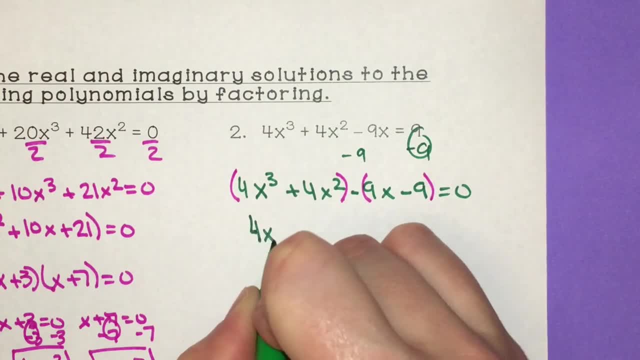 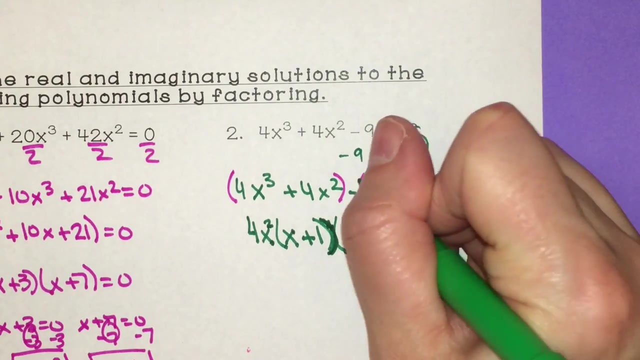 factor out This first one. I can factor out a 4x and I'm left 4x squared. sorry, I'm left with x plus 1.. I want a plus in between. I'm just going to rewrite that plus. I wanted this, did not take that into account. I wanted this negative inside the 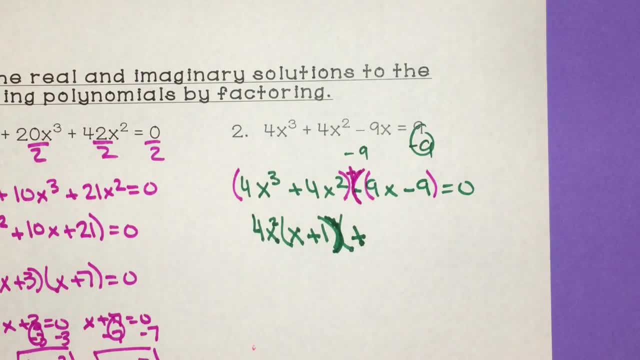 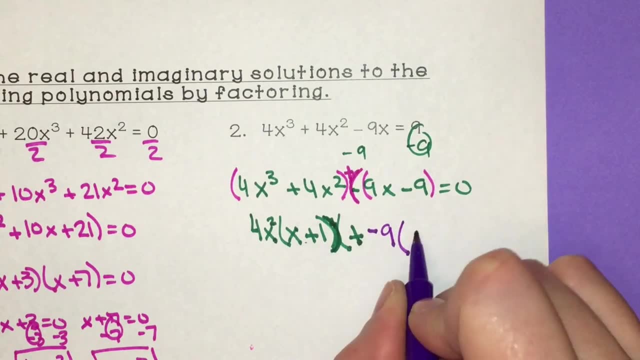 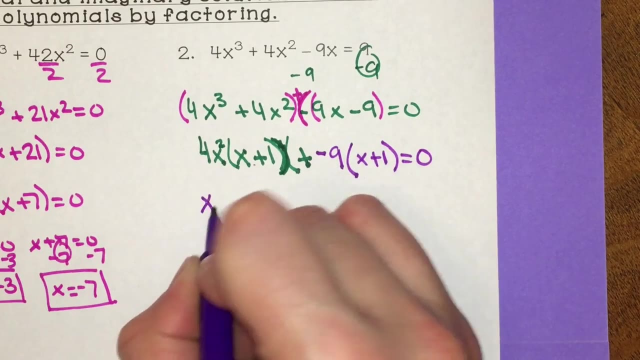 parenthesis and I put plus in between. Alright, to get what's in the parenthesis to be the same, I'm going to factor out a negative 9. Then I'll be left with x plus 1 in my parenthesis. So my new greatest common factor is x plus 1.. So factor that one out. 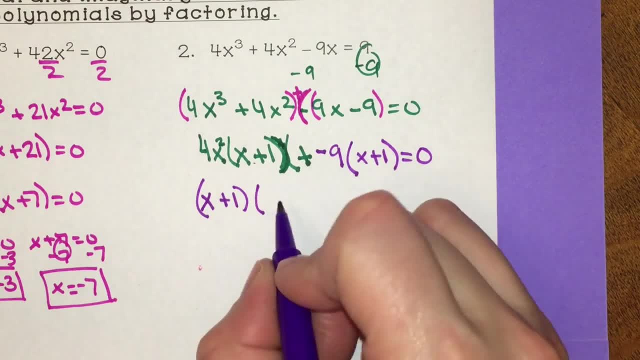 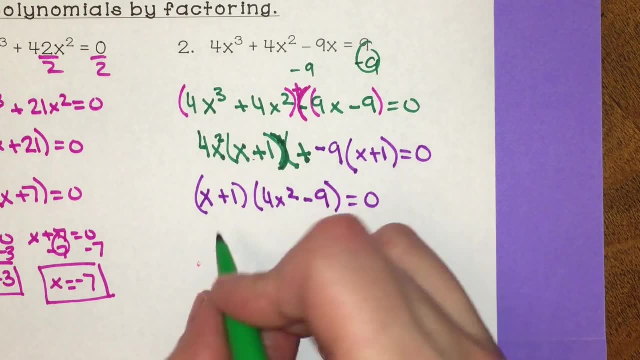 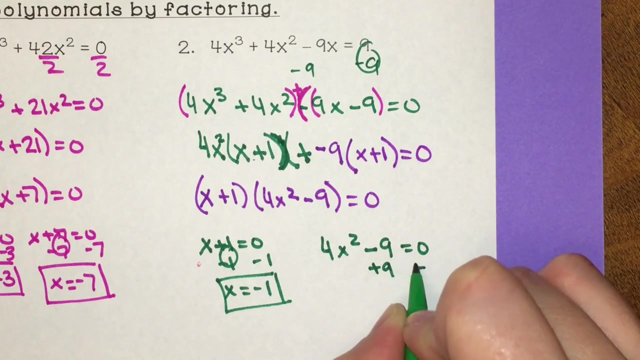 Times. here we have: 4x squared minus 9 equals 0.. Okay, so x plus 1 equals 0.. Subtract 1 on both sides and x equals negative 1.. Over here, 4x squared minus 9 equals 0.. Add 9 to. 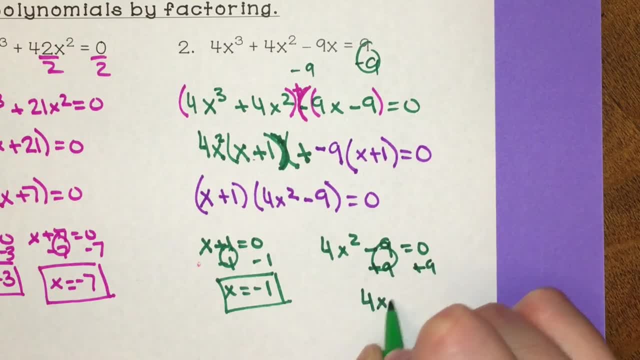 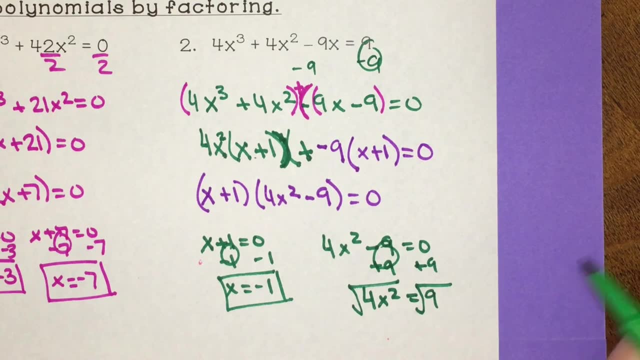 both sides and we get 4x squared minus 9 equals 0.. 9 is equal to 9.. Take the square root of both sides. Well, square root of 4x squared is 2x equals. we have to take into account both positive and negative, because x was squared. 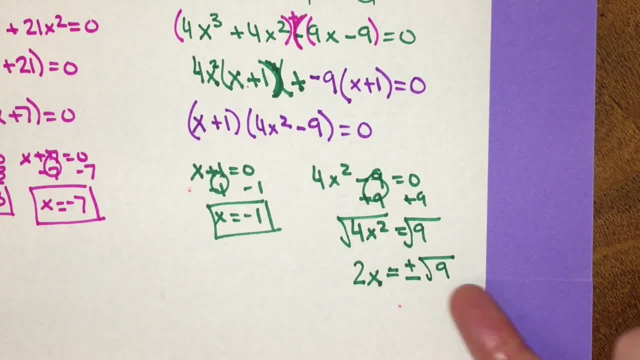 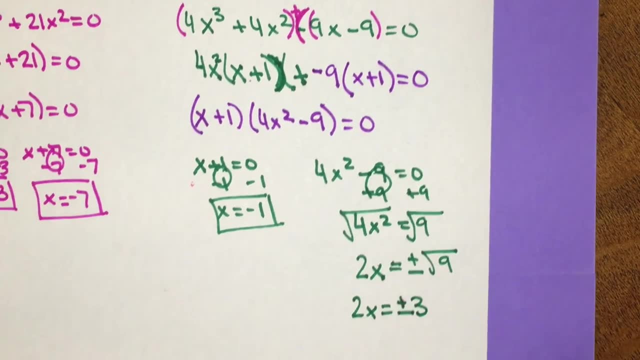 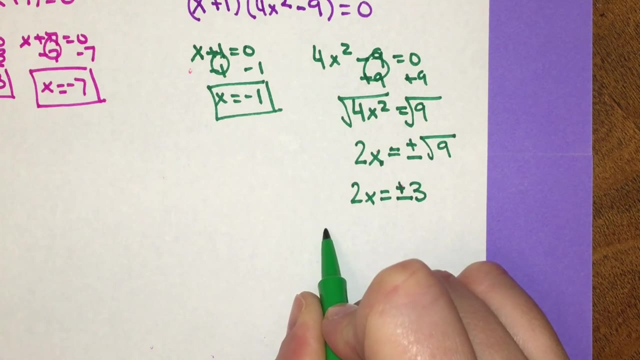 We have square root of 9.. And while the square root of 9 is just 3, so we have: 2x equals positive and negative 3.. So here I'm going to do each of these, I'm going to do each individually. I'm going to say that 2x equals 3.. Divide both sides. 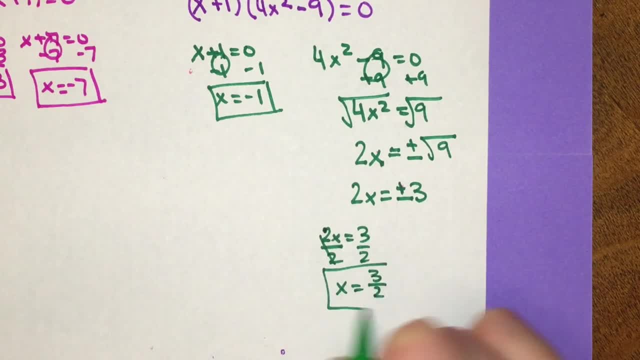 by 2. We get x equals 3 halves And 2x equals negative, 3. Divide both sides by 2.. And x equals negative 3 halves. So positive, negative 3 halves and negative 1.. Alright and number. 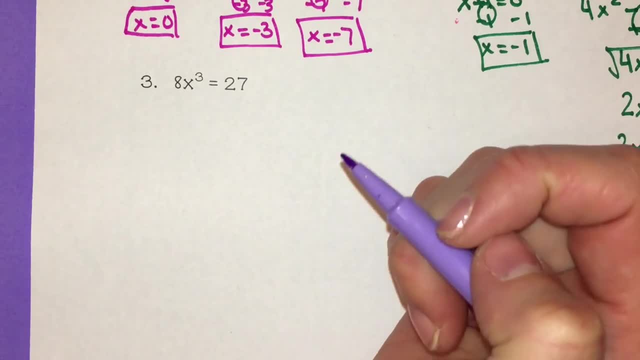 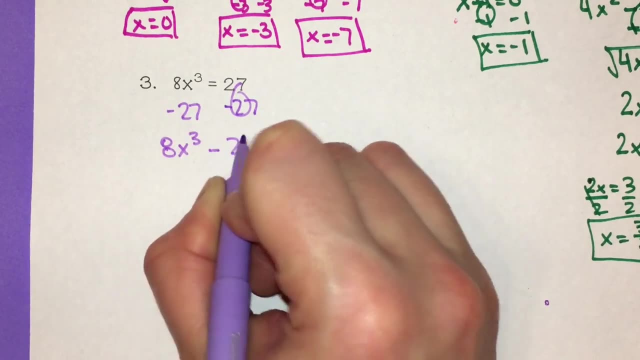 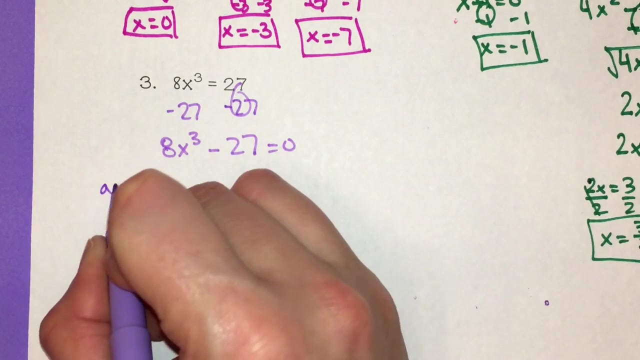 3.. Okay, so I'm going to subtract 27 on both sides and get 8x cubed minus 27 equals 0.. Okay, so this is difference of cubes. I know that a is equal to 2x, b is equal to 3.. So 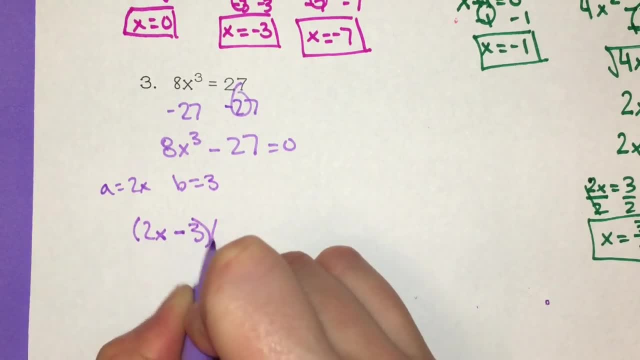 we have 2x minus 3 times my 8x. divided by 2x times 2x equals 1.. And I'm going to subtract 27, a term squared well, 2 times 2 is 4 and x times x is x. squared plus 2x times 3 is 6x. 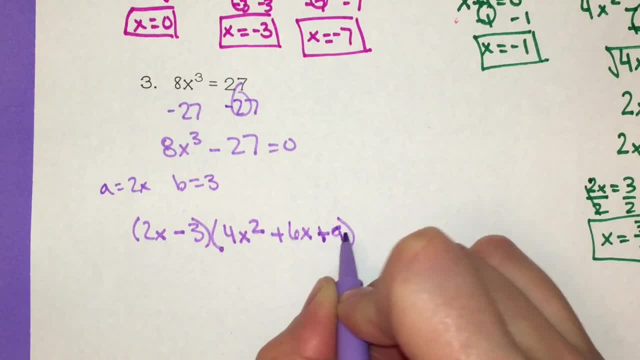 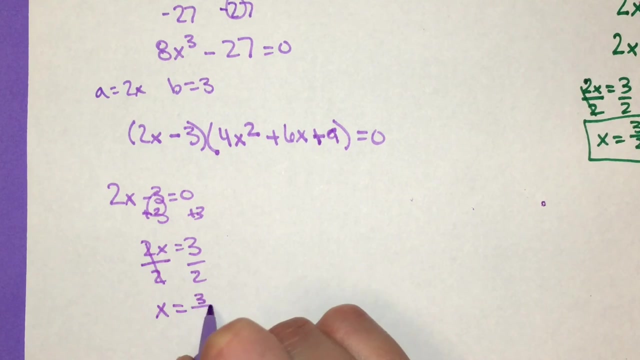 plus 3, squared is 9, is equal to 0. So here we have: 2x minus 3 equals 0. Add 3 to both sides, we get 2x equals 3.. Divide both sides by 2 and x equals 3, halves, Alright, so can. 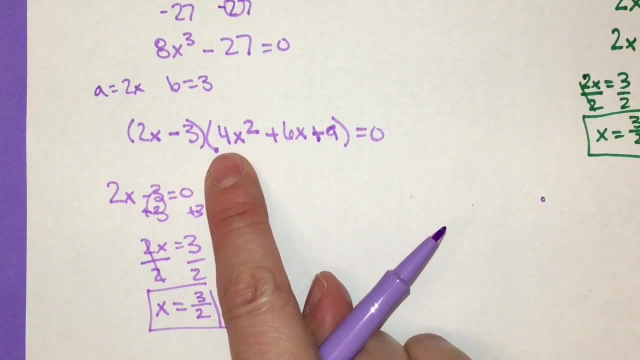 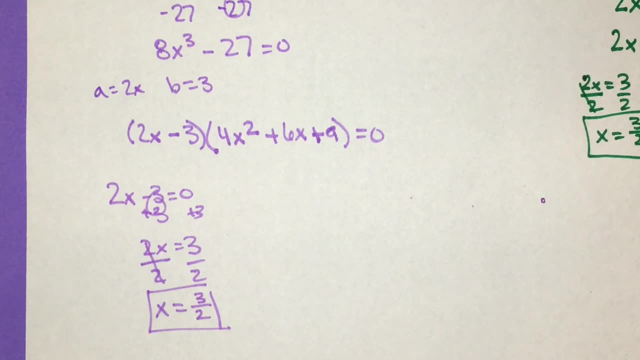 we multiply anything. oh see, we have. multiply anything to get 4 times 9, which is 36.. Add anything to get 6.. 6 times 6.. Well, we can always do that quadratic formula: A equals 4, B equals 6, C equals 9.. So you can do negative B, which? 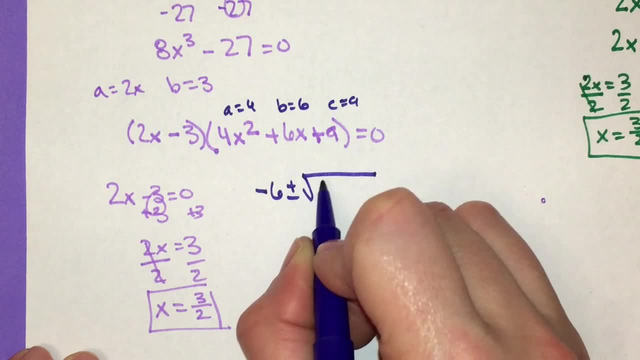 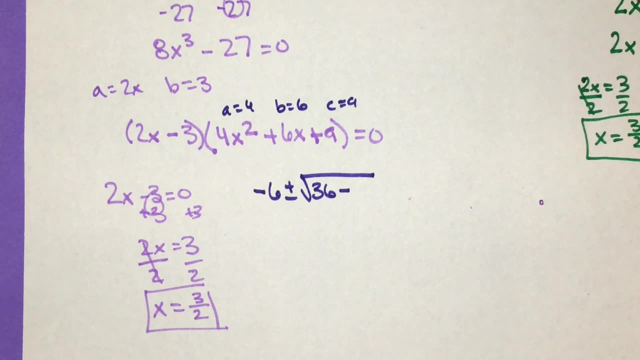 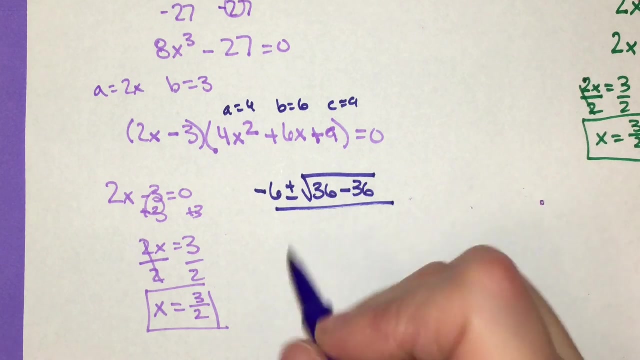 is 6 plus and minus. the square root of 6 times 6 is 36 minus 4 times A, which is 4 times C, which is 9, is 36 divided by 2 times A. So there are multiple ways to do this. one, 2 times 4, which is 4, gives us X equals negative 6.. Well, 36 minus 36 is.